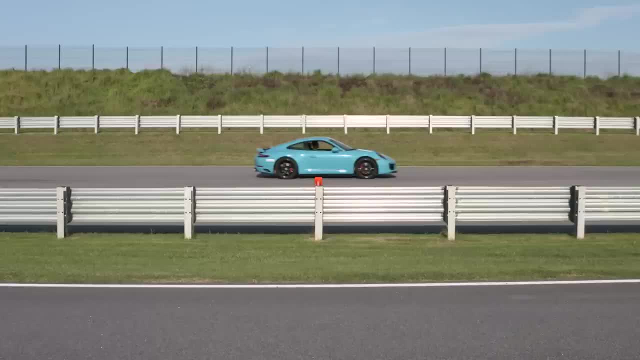 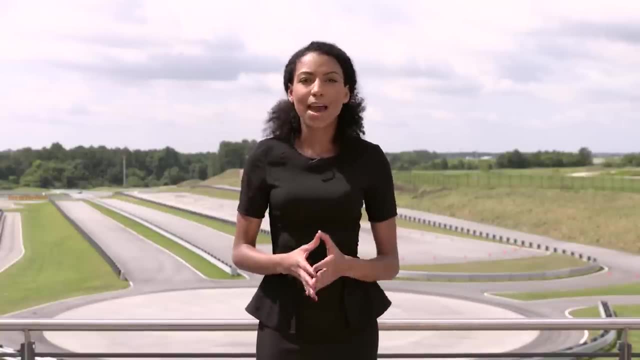 The SI unit for speed is meters per second. It's a scalar quantity, meaning it only has a magnitude. For scalar quantities such as speed, the direction the object is moving in doesn't matter If the car keeps moving just as fast as it was before. 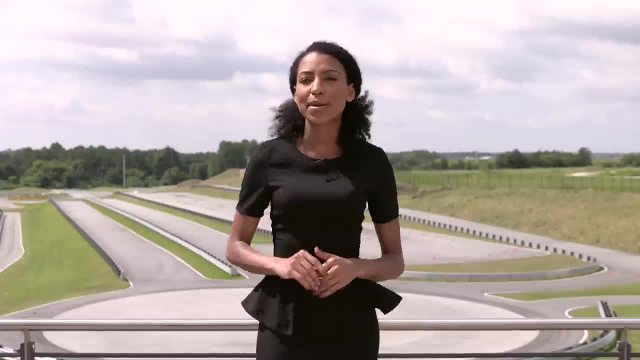 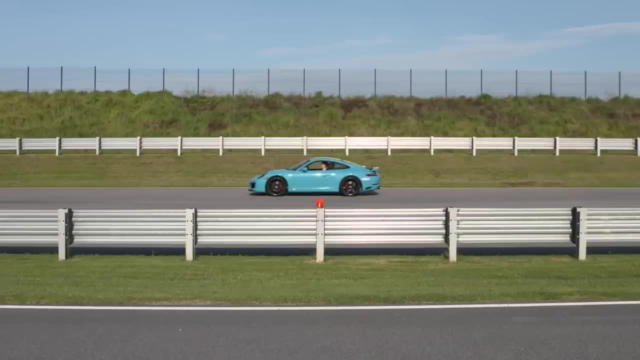 except this time it's going the opposite direction. its speed still remains the same. Just because the car is moving in the opposite direction doesn't mean the speed is negative. Speed will always be a positive value. We calculate the average speed of an object. 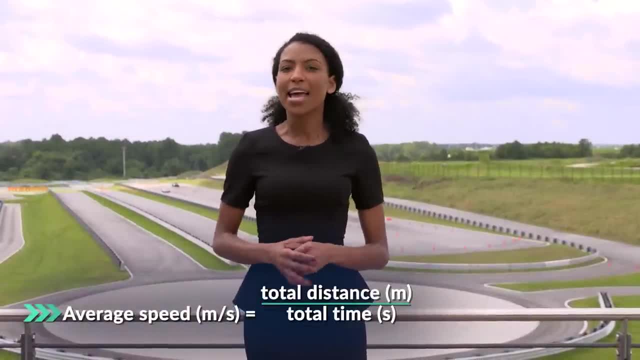 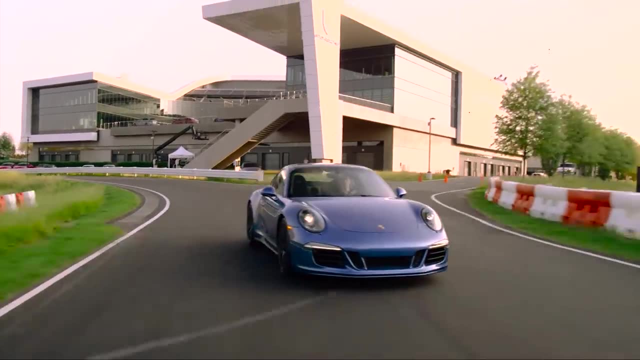 by using this equation, The average speed in meters per second is equal to the total distance traveled in meters divided by the total time taken in seconds. Let's work through an example. When a car makes a lap around the track, we can calculate its average speed. 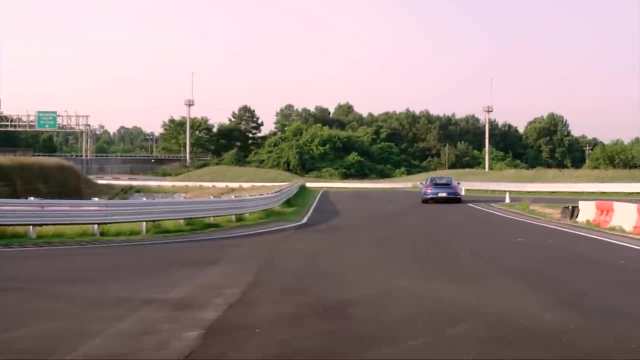 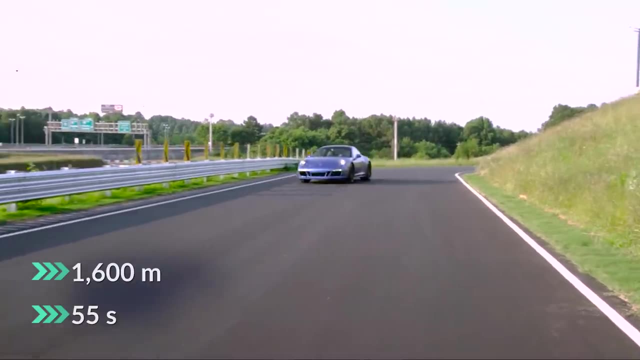 using the distance it traveled and how much time it took. One lap around this track is 1,600 meters and the time it takes this car is 55 seconds, So the average speed was 1,600 meters divided by 55 seconds. 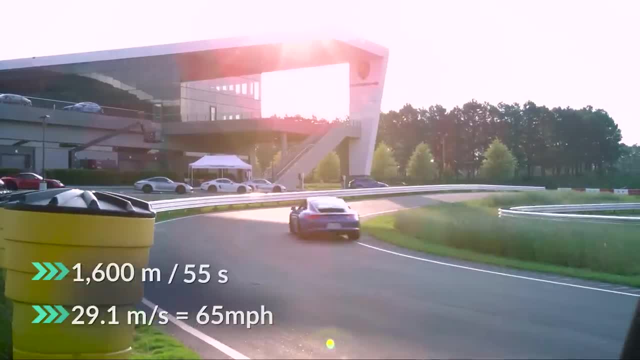 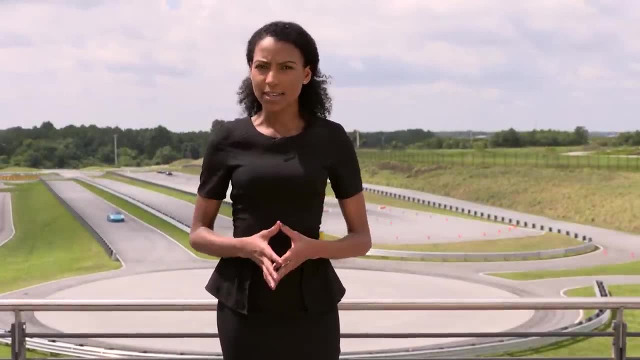 which is 29.1 meters per second. That's pretty fast. Okay, we've talked about speed as a scalar quantity. What about velocity? Velocity is a vector quantity. It means it not only has a magnitude, but it also has direction. 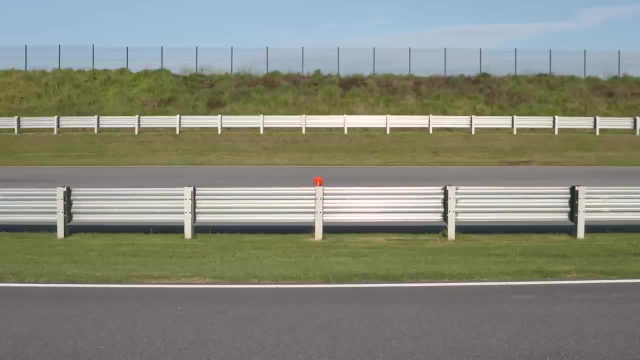 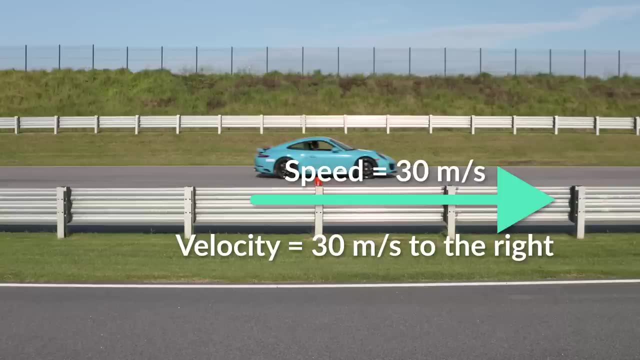 The SI unit for velocity is also meters per second. so when a car speeds past again, its speed is 71 miles per hour or 30 meters per second, but its velocity is 30 meters per second. going right, Average velocity is an object's change in position. 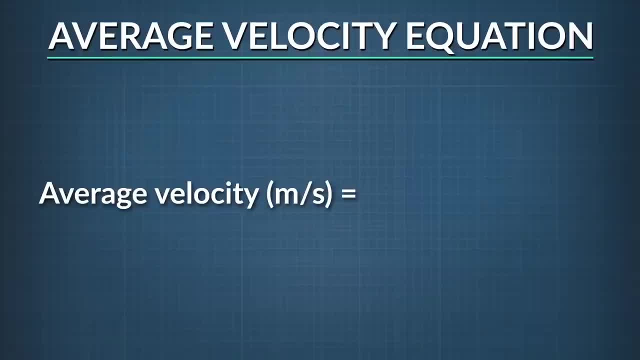 or displacement over change in time. We can calculate it using this equation: An object's average velocity in meters per second is equal to its change in position or its displacement in meters divided by the change in time in seconds. When solving this problem, 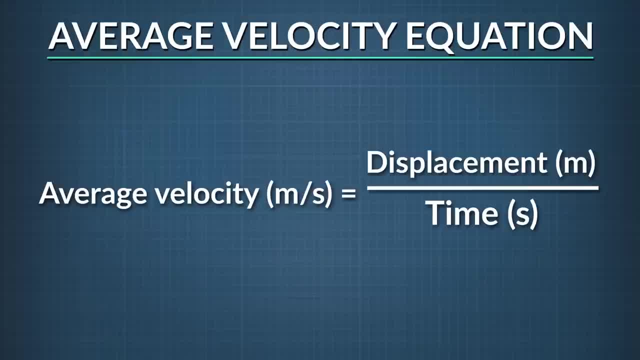 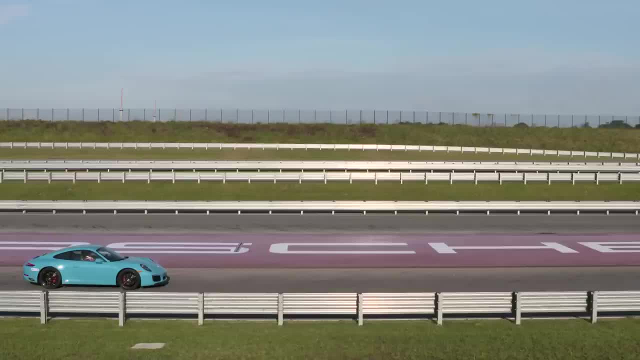 of velocity, it's important to establish a frame of reference. Let's go to the track for an example. Say that right is the positive direction and left is the negative direction. A car is stationary at our origin point, point A facing right. 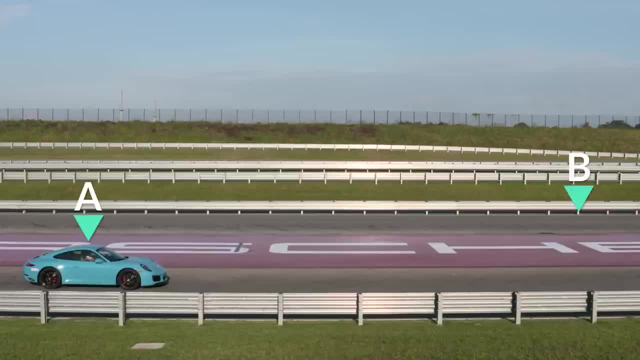 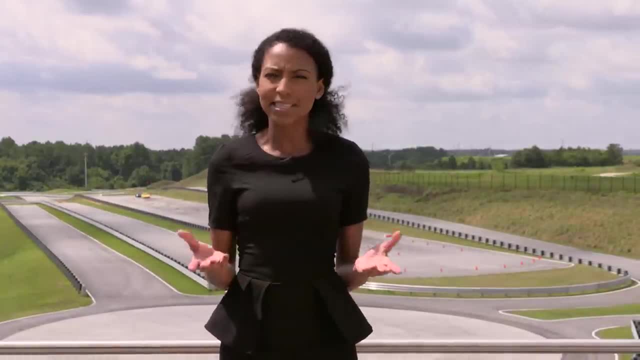 It's going to speed towards point B and turn around to stop halfway back to point A at point C. Would the average speed and the average velocity of the car over this journey be the same? Well, there's only one way to find out. 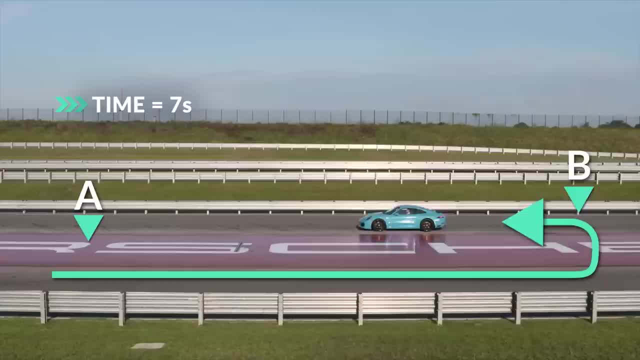 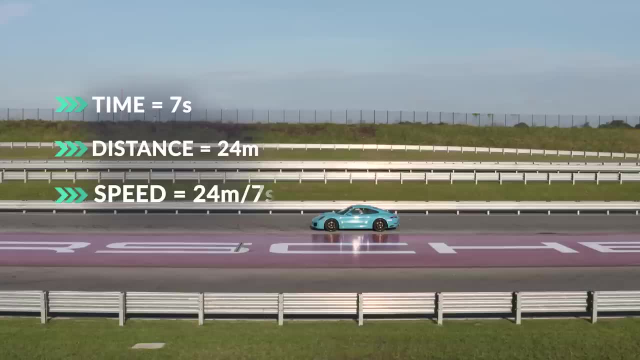 It took the car seven seconds to complete its journey. The total distance it traveled was 24 meters. This means that the average speed was 24 meters divided by seven seconds, which is 3.43 meters per second. However, the total distance traveled by the car, 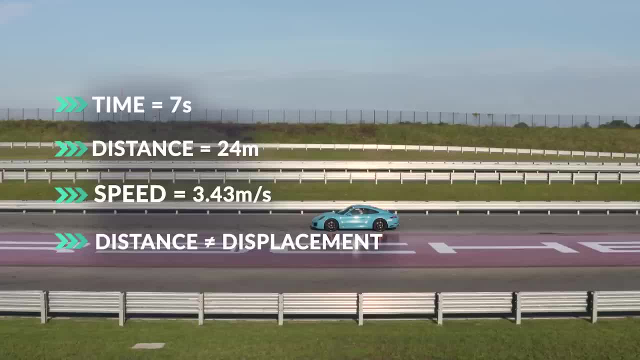 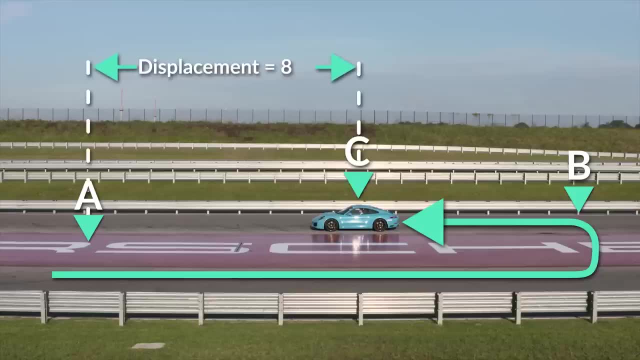 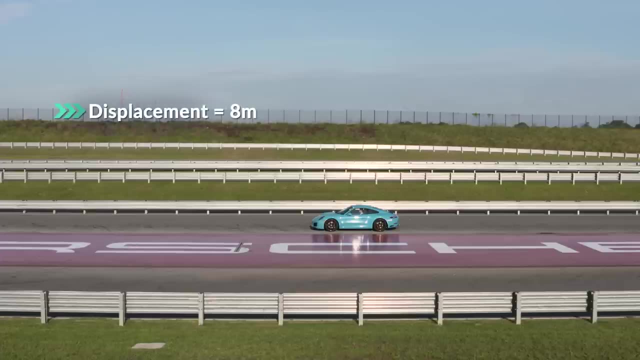 is different from the total displacement. The car's displacement only takes into account the point-to-point difference in meters between the origin and the final destination. The displacement from point A to point C is eight meters. This means that the average velocity of the journey is positive eight meters. 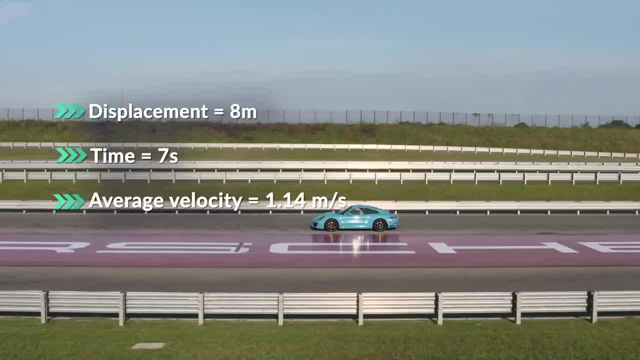 divided by seven seconds, which is positive, 1.14 meters per second, or 1.14 meters per second to the right. So it's possible for the average speed and the average velocity to have two separate values even for the same journey. 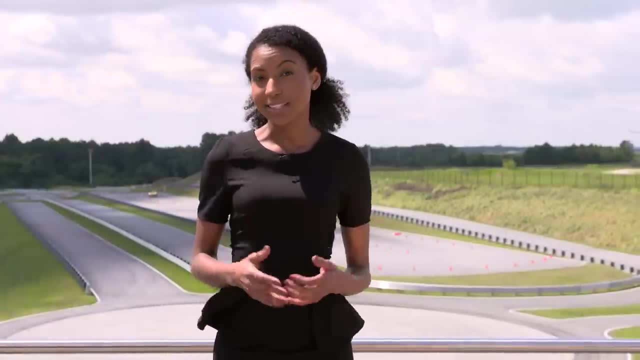 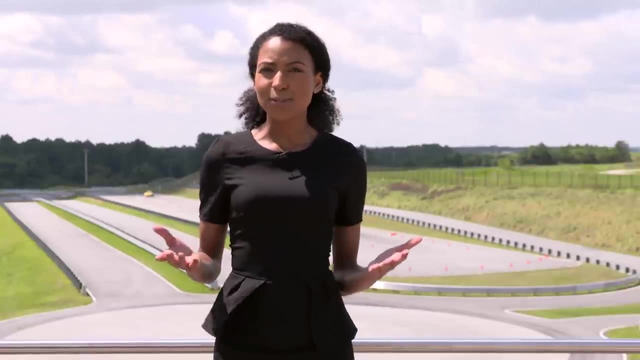 To recap, speed is a scalar quantity, which means it has magnitude only. Velocity is a vector quantity, meaning it has both magnitude and direction. But how are we supposed to know which direction is positive And which direction is negative? Good news, it's our choice. 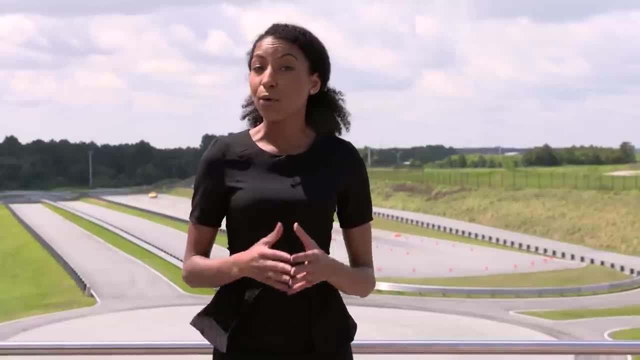 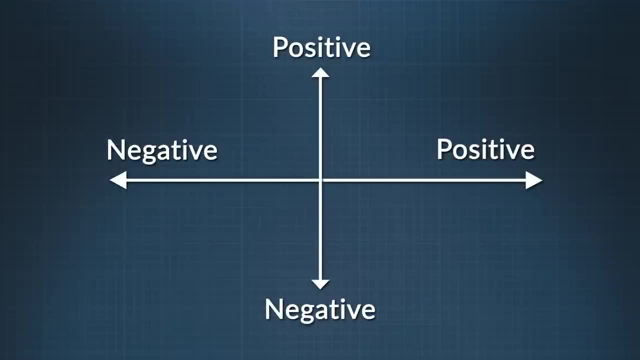 We pick our own negative and positive directions. So when you're given a problem to solve, indicate which direction you've picked to be positive. Whatever answer you get should reflect that choice. We usually treat right and up as positive and left and down as negative. 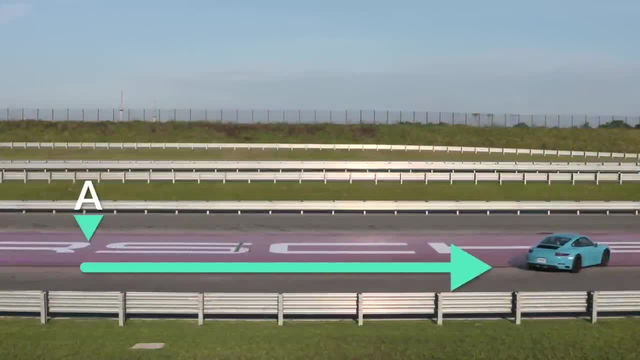 So when the car was going from point A to point B, it was traveling the positive direction, because we've designated right as the positive direction. If the car went from A to B in four seconds, then its average velocity was 4 meters per second. 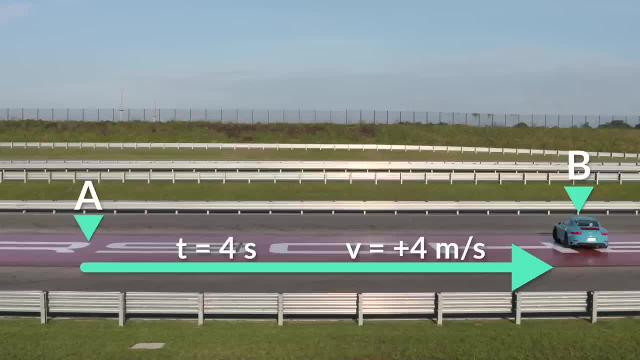 going in the positive direction, But when the car was going from point B to point C it was facing the other way. If it did so in three seconds, then it had an average velocity of 2.67 meters per second in the negative direction. 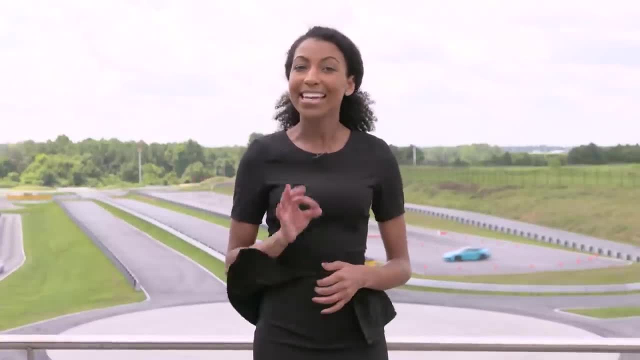 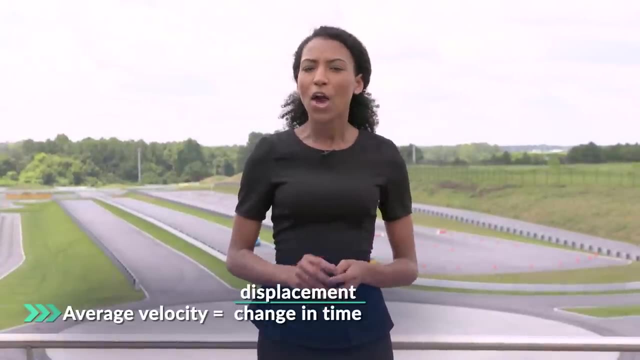 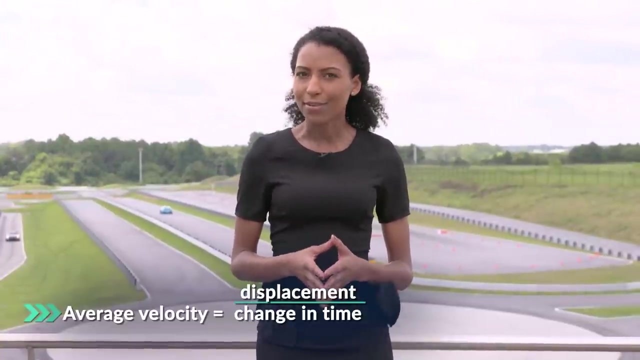 Now let's talk about the difference between average velocity and instantaneous velocity. Average velocity, as we've been discussing, is the displacement divided by the change in time. We calculated the average velocity of the car going from point A to point C, But what about the journey itself? 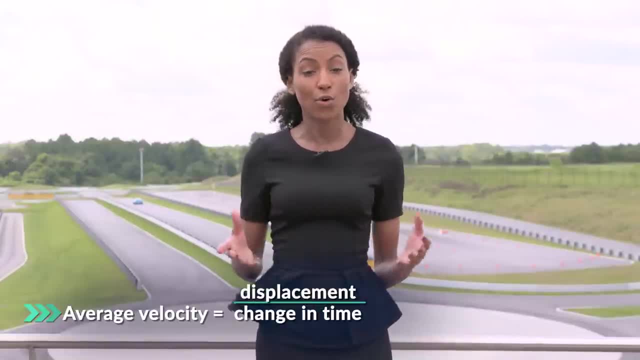 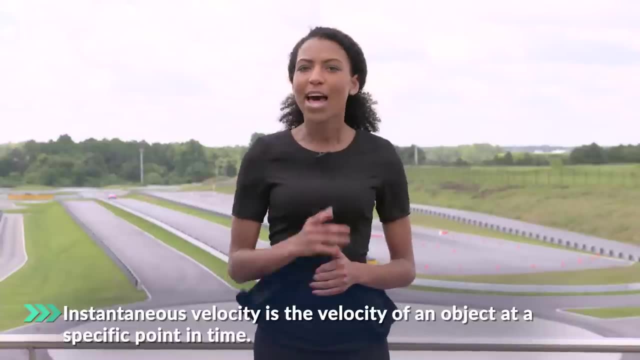 The average velocity tells us the overall velocity over the course of the entire journey. The instantaneous velocity is the velocity of an object at a specific point in time. Let's look at the car as it was starting to accelerate and freeze it right there At the time: 0.5 seconds. 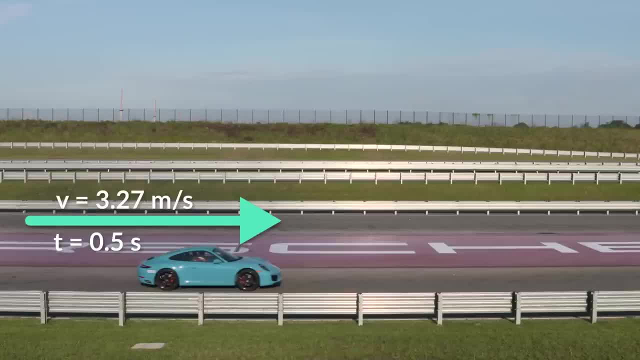 its instantaneous velocity is 3.27 meters per second. to the right. As the car speeds up, its velocity increases. What if we sped up to right here at 1.5 seconds? Its instantaneous velocity is now 9.81 meters per second. 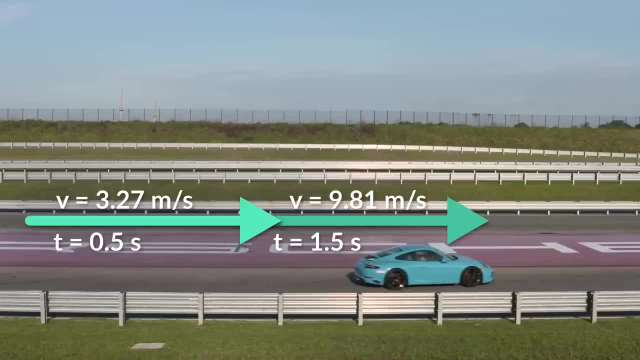 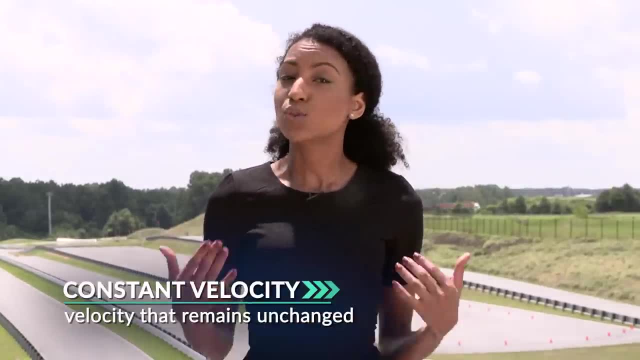 to the right. Remember: the instantaneous velocity is the velocity of an object at a specific moment in time. Another important term to know is constant velocity, which is what we call unchanging velocity. Okay, so we've learned what velocity is, whether it's average, instantaneous or constant. 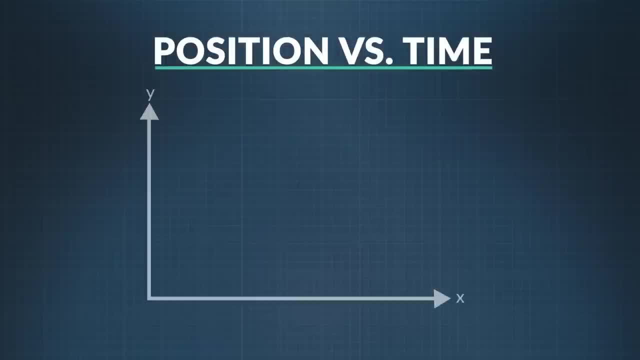 But how do we represent it? If we have a position-time graph, we can use it to calculate the velocity of an object at a specific point in time. We can use it to learn about an object's velocity In a position-time graph. 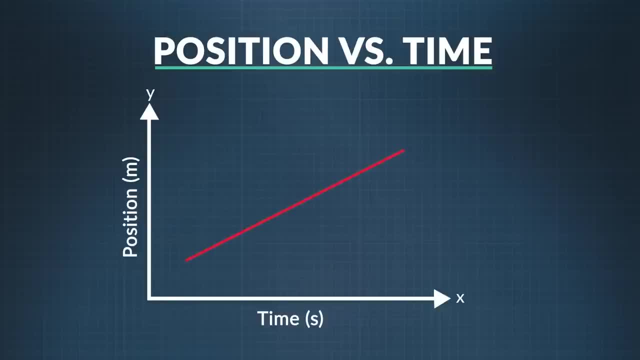 the time elapsed will be shown on the x-axis and its position shown on the y-axis. This graph shows a constant velocity which, on a position-time graph, looks like a straight line. By looking at the slope of the line in a position-time graph, 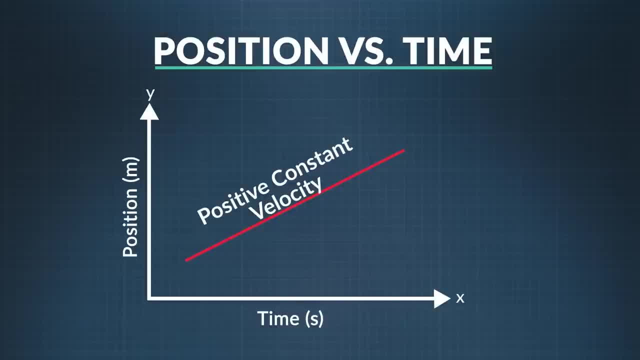 we can learn about an object's velocity. It makes sense that this object is moving at a constant velocity because the slope of the line is not changing. So we can calculate the velocity of an object at a specific point in time. We can calculate the constant velocity. 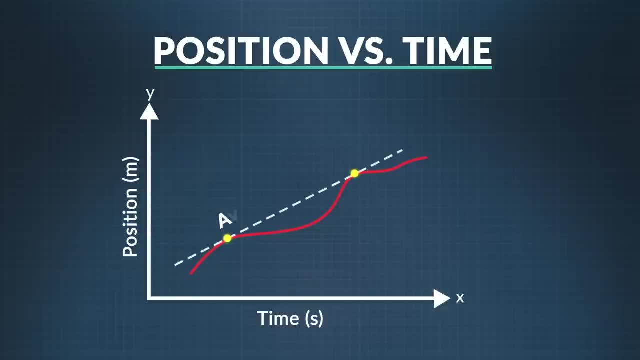 by finding the slope of this line. If the velocity wasn't constant, we can calculate the average velocity by drawing a line between two points in time and find out the slope of that line If we want to know the instantaneous velocity or our velocity at a given point in time. 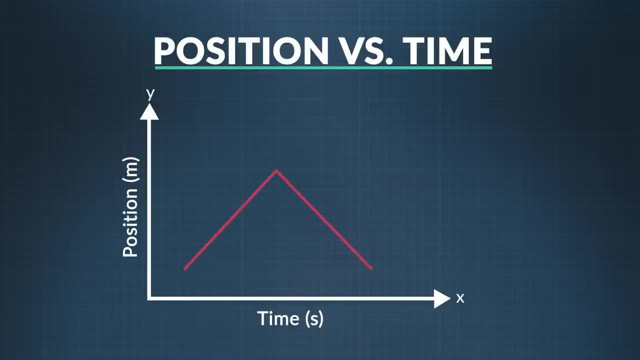 we can draw a tangent line from that point in time and find the slope of the tangent. We can also have graphs that look like this, with the line going up and down. Notice I'm moving in the positive direction, away from my origin. This would be me moving at a constant velocity.